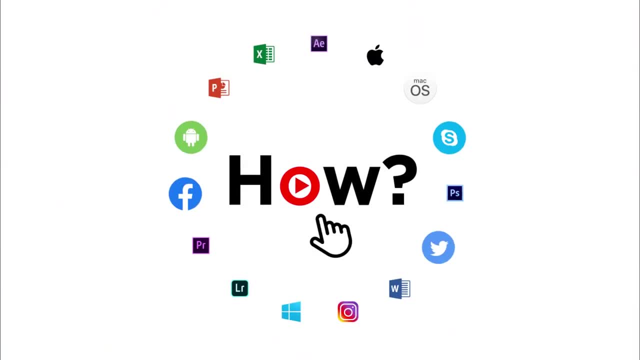 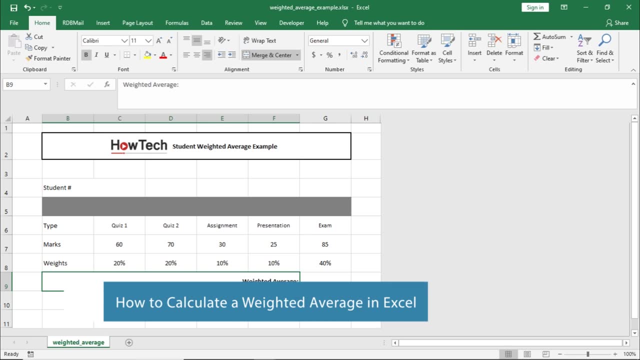 Hello and welcome to HowTechTutorials. In this video we will teach you how to calculate weighted average in Excel. To calculate weighted average, a predetermined weight is assigned to each number in the data set Over. here you can see the marks: a student 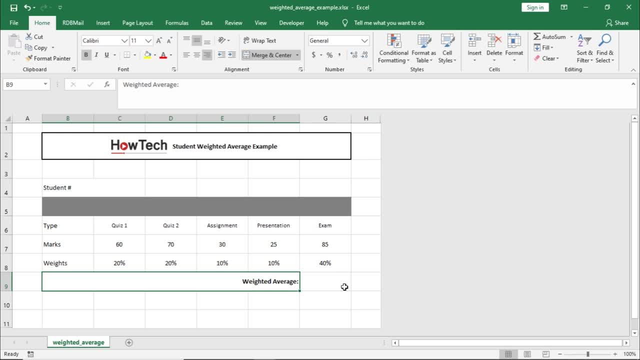 has achieved during a semester, against each quiz, presentation, assignment and exam. In this scenario each criteria is provided a weight. So, for example, quiz 1 here is worth 20% of the overall percentage. Therefore, in our calculation we will have to consider: 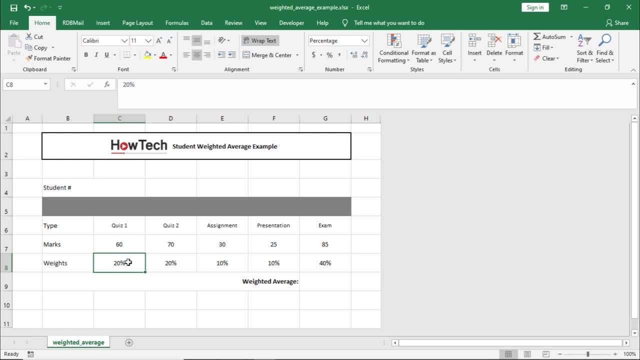 the weights assigned against each criteria to calculate the overall percentage at the end of the semester. To calculate weighted average, each criteria is multiplied with its respective weight. The result for each criteria is then added up and divided by the sum of all weights. In Excel, this can be done by using the SUMPRODUCT. 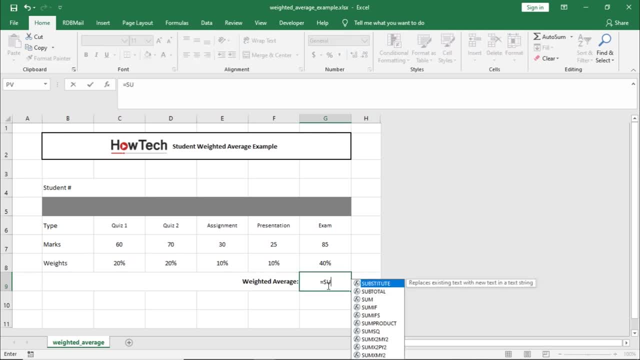 and SUM function. Let's type in the equals to sign, followed by writing SUMPRODUCT, and brackets open Over here. you can see that the SUMPRODUCT function multiplies multiple arrays, So let's select the entire range of marks obtained. Now let's enter a comma and then select the 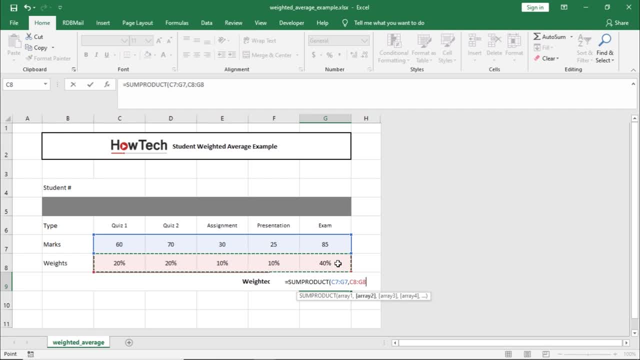 range of weights assigned. This is essentially multiplying each mark obtained with the weight assigned for each criteria and then adding up the result for all five criterias. here Let's close the brackets, and now we will enter the divided by sign. After that, let's enter. 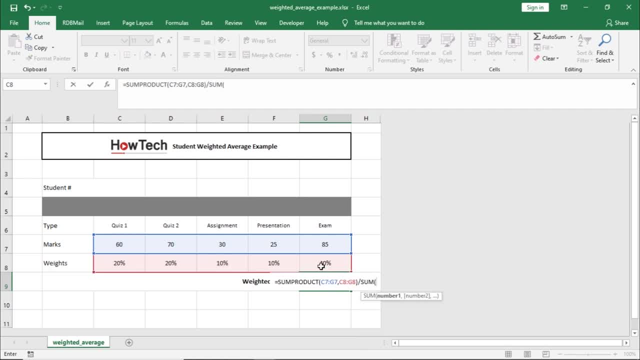 SUM, followed by brackets open. Now let's select all the weights Over. here. we are basically dividing the output we get from the SUMPRODUCT function with the sum of all the weights in this data set. Once we hit enter, Excel will calculate the. 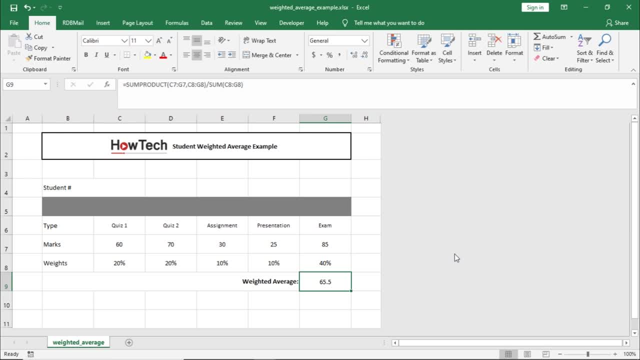 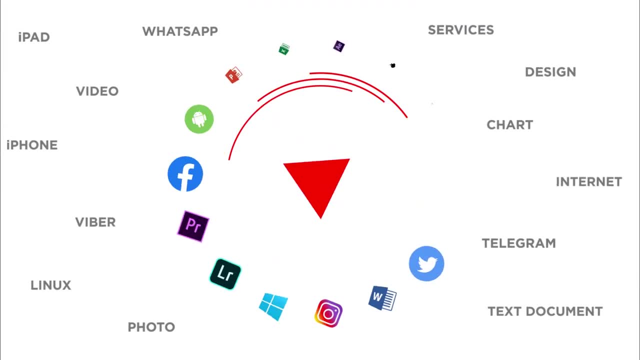 weighted average score over here. That's all. Is there any Excel function you would like to know more about? Let us know in the comments below. Thank you for watching. If you liked this video, don't forget to give it a thumbs up. 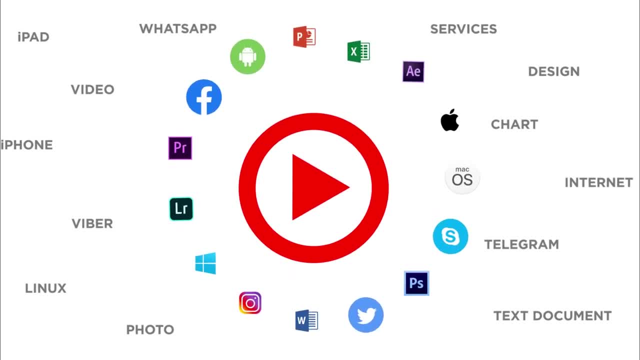 and subscribe to our channel, and make sure to press the bell button to be the first to know about our new videos.